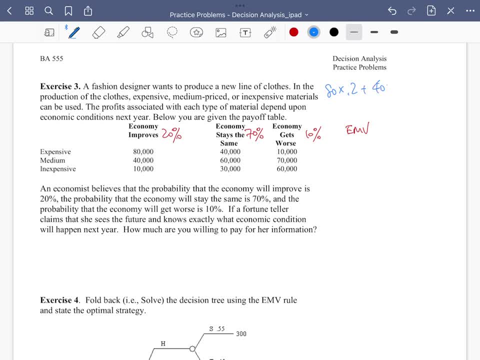 going to write down here: right, and that's going to give us 45k. I'm going to write down: here is 45k for expensive material and for medium material is going to be 47k and for the inexpensive material is going to be 29k. well, so now the options are very clear. so, based on the EMV, we know that she 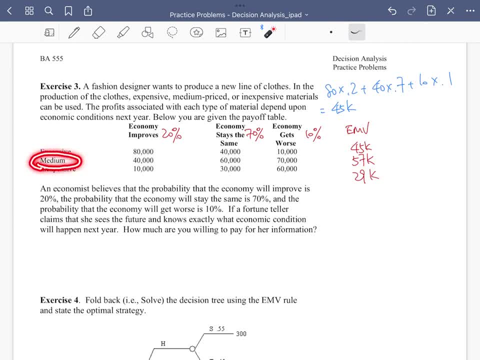 is better off if she use medium materials because that's going to give us the highest EMV right EMV. without any additional information. any additional information, just use the information provided by the economist. the EMV is going to be 47k when she uses medium materials. 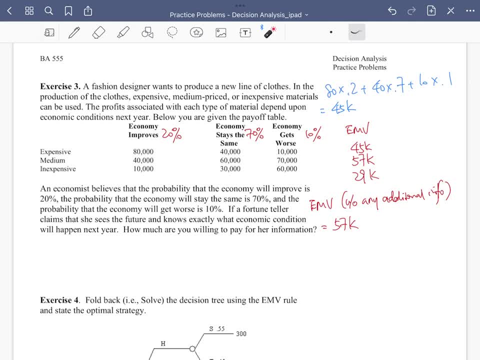 you okay? next, there's a fortune teller and she sees the future and knows exactly what economic condition will happen, and how much are you willing to pay her for this perfect information? well, if the fortune teller knows the economy, whether it improves or not based on that piece. 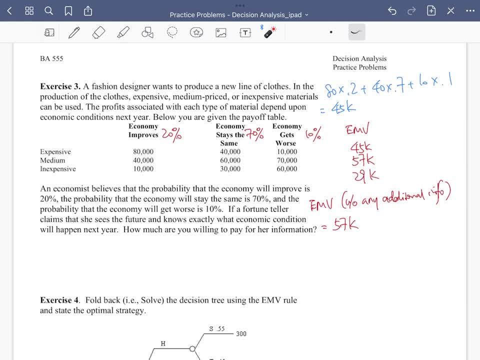 of information we can tell the fashion designer what option she should choose. for example, if the economy improves, clearly, out of the expensive material, she's going to be better off if she use medium materials and not the expensive pieces, since if she use the clothes of an expensive or 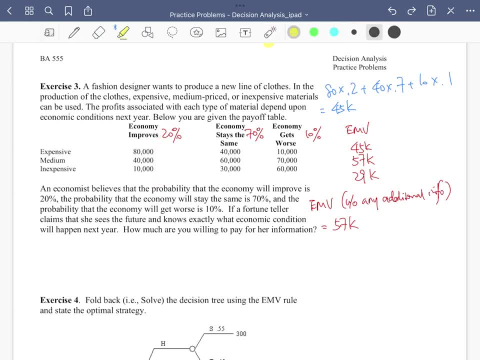 medium, inexpensive clothing. our fashion designer should choose the expensive one because that's going to give her the highest profit. if the economy stays the same, she should choose that medium clothing. if the economy gets worse, she should also choose the medium clothing. so that means the highest payoff for economy improves is 80k, economy stays the same as 60k and if the 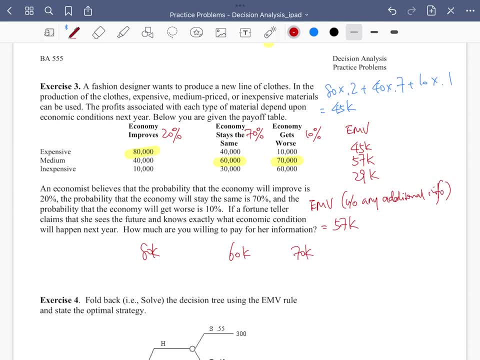 that 70k. right, we also have their respective probability because there's a 20% economy is gonna improve. so that means 80k multiplied by 20 and 70% of time, the highest profit this fashion designer is gonna make is gonna be 60k. 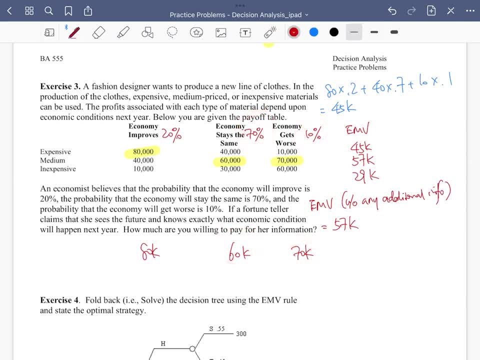 and 70k for 10% of time. so, based on those information, we can calculate EMV with perfect information, perfect info, and that's gonna be 80K multiplied by 20 plus 6 K, multiplied seven point seven plus 70K, multiplied by 10 percent of 0.1, so that's gonna give us EMV 65K, right? so 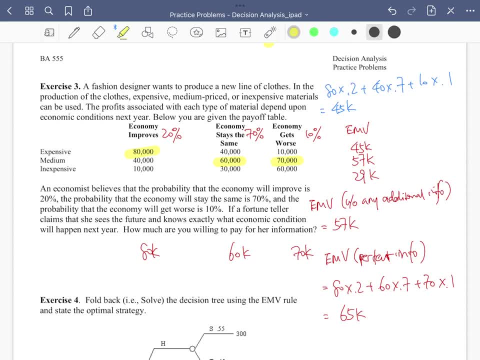 what we're to do right now is, without the fortune-tellers information, the fashion designer is able to have a profit of 50K and 70% of time, of 10% of time, right and before it's too decades away- and 57k. with that piece of information, she is able to make even more 65k. so how much are you willing? 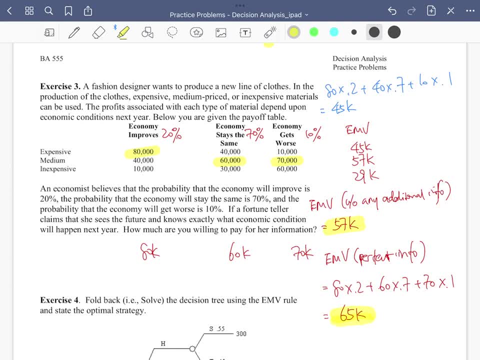 to pay. are you willing to pay, say, ten thousand dollars more well, i don't think so, because without a fortune teller's help she was already able to make 57k, and the maximum amount of profit she's going to get with that, additional information from the fortune teller is only the difference. 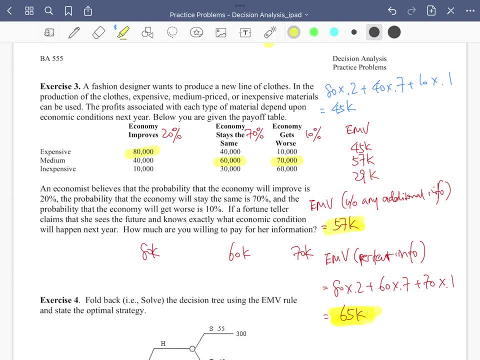 between those two is only eight thousand dollars, so the fashion designer should not be willing to pay for anything more than eight thousand. so i'm gonna write it down: not more than eighty thousand dollars, right, okay? okay, hopefully this part is clear and let's move on to question four. okay, 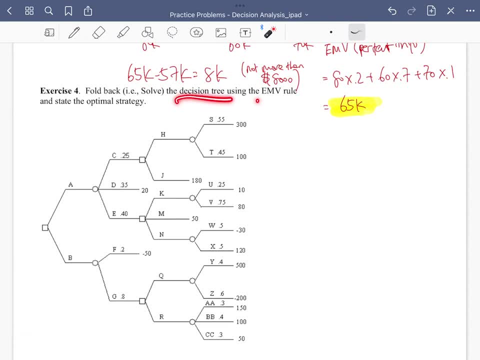 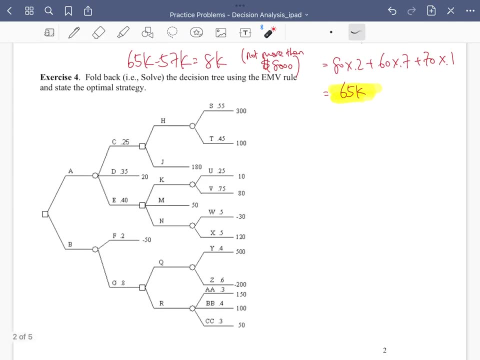 so we'll be have here is: we have a decision tree and we want to use the mv rule to state the optimal strategy. okay, you probably have seen this kind of trees in the slides, in the videos. okay, so what we want to do here is to solve the tree. we go from the right to the left, so i'm going. 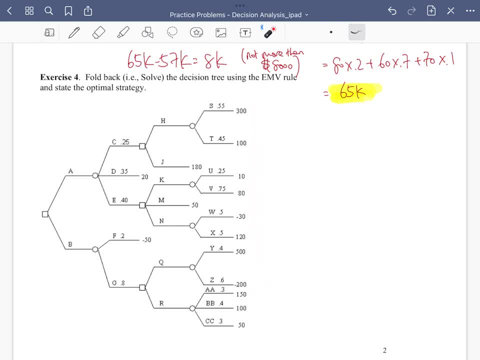 to start with here, the very last end, there are different decision nodes and there are chance nodes. okay, i'm gonna just quickly write it down here: this is a decision node, so decision node, we're gonna make a decision, we're gonna decide which one, we're gonna choose, which action to take, so that you really involves. 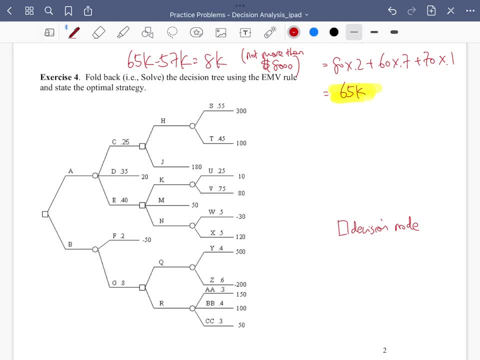 choosing the branch that leads us to a higher cmv and a circle represent chance node. chance node has probability associated to different branches. we want to calculate the expected emv at a chance node. i'm going to show you what exactly i meant, so let's start from here. the first node i see is a. 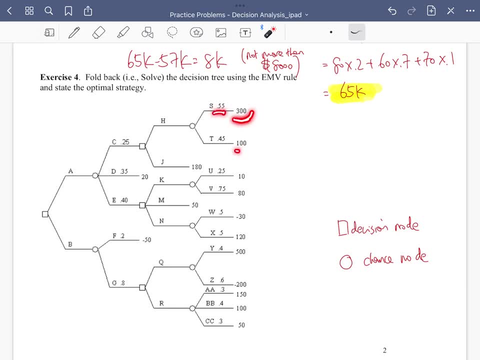 chance note: 355 percent of time. 100 dollars payout 45 percent of time. so this is a chance note. we are going to calculate the emv at this chance node. so let's do that. it's going to be 300 times 0.55 plus 100 times 0.45, right? if you do that, that's going to give us 210, okay, 210. 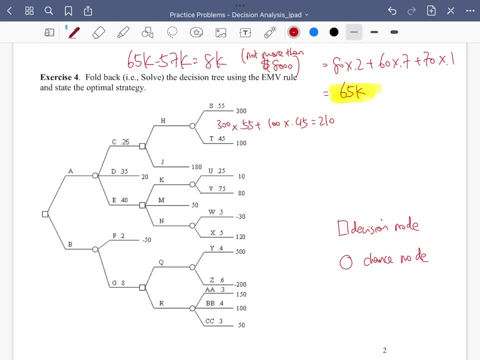 so i'm going to do is i'm going to write it out here is 210, the payoff is 210. i'm going to erase this one, okay, and we move from the right to the left. so this is 210. this branch leads to emv of. 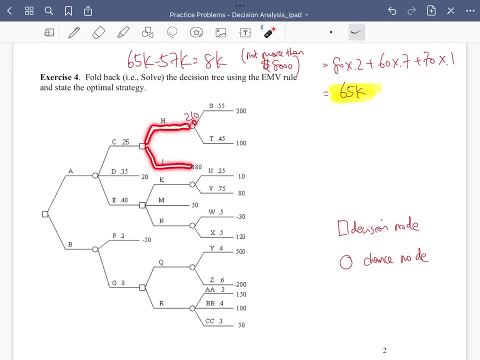 210 and the next branch leads to emv of 180 and at the square node, the decision node, we're going to decide which path we're going to take. i'm going to take 210 going through path 8. i'm going to take a payoff- 180 going path j. certainly we want to go with the 210. so 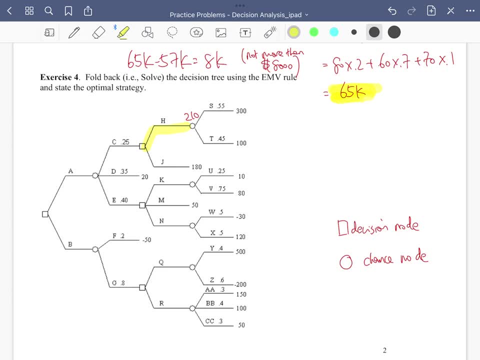 take 210, right. okay, we're going to move on to the uh, to the next cluster of nodes, so we do the same thing here. so again, it's a circle node. we're going to calculate the emv here. so you can do that. i've already done it. the emv is 62.5 and same goes here. you can calculate the emv as well. 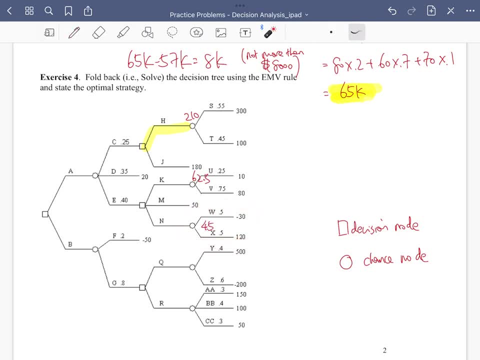 and that's 45, right? so a decision note three branches: 62.5 or 50 or 45. so we certainly want to go with the 62.5. so that's going to be here, right, 60.5, okay. so we are pretty much, uh, completed with this big branch. 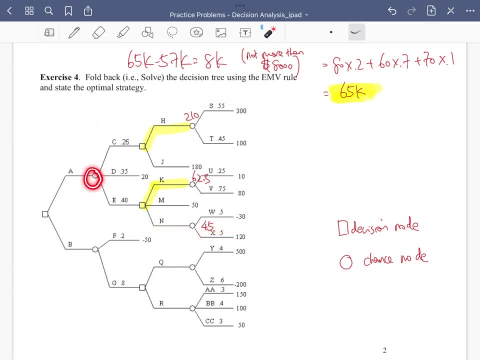 let's take a look. so this is again a circle node. so we want to calculate the emv here. so 25 of time give us 210 because we take the path of h. so this one and this here is 210. i'm going to write down. 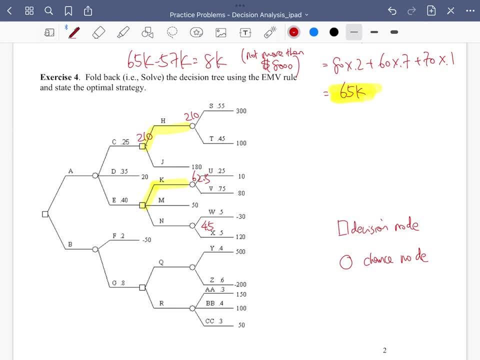 here 210 and we're going to take this path of 62.5. so over here is 62.5, right. so we want to calculate the chance. no emv, okay, that's going to be 210 multiplied by 25 plus 20 and 35 and 62.5, 40 percent of time. 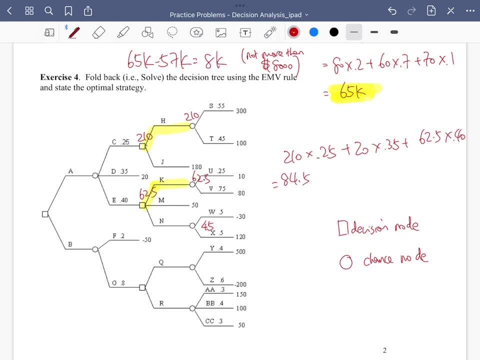 right, that should give you 84.5. so i'm going to write down here, at this circle node, the emv is 84.5, right, okay, so i'm going to move on to the next lower branch here. so again it's a chance node. we calculate the emv and this is actually uh 80 here. so for our second chance node, 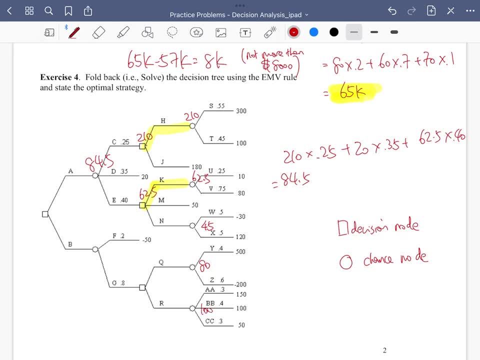 the emv is 100.. well, comparing 80 branch versus 100, we're going to go with this branch, right? so i'm going to highlight it here, okay, and i'm going to carry over their emv 100 here, Okay. so now another circle node. 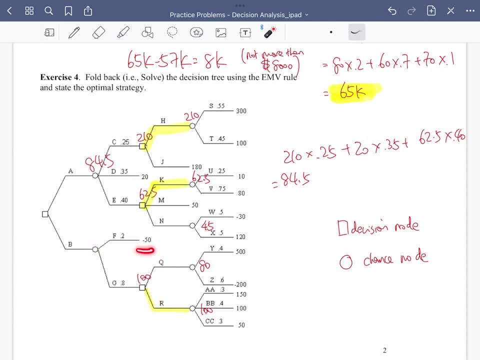 we can calculate the EMV here. So negative, 50, 20% of time, 100, 80% of time, So the EMV can be calculated and that's 70.. Okay, so we're almost done here. 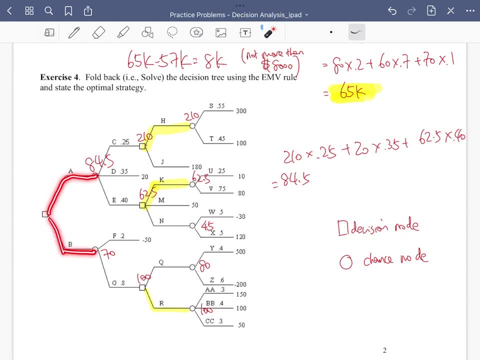 Last decision, node 84.5 or 70. We certainly want to prefer the higher one, so that's gonna be 84.5, right. What's the final decision then? The first decision we do is we choose A which allows us to go through this route. 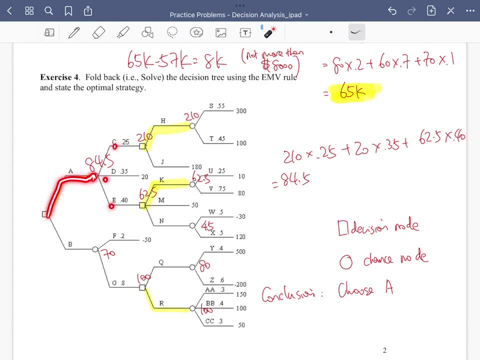 Okay, and we are facing three choices: C, D, E. If C happens, we are gonna choose H. right, We're gonna choose H. We're gonna get a payoff of 210.. Okay, if D happens, we don't have to do anything. 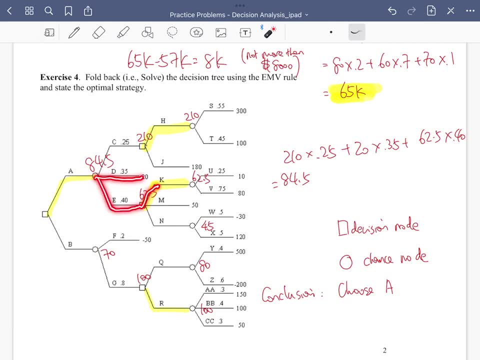 If E happens, we are gonna choose K and we're gonna end up with 62.5, right, Okay. so if C happens, we choose H, If E happens, we choose K, right, And final expected monetary value for the entire tree.